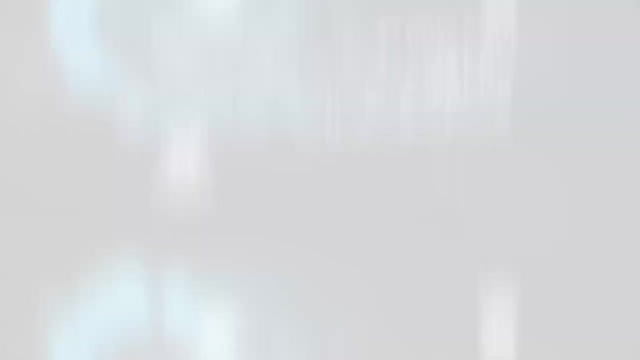 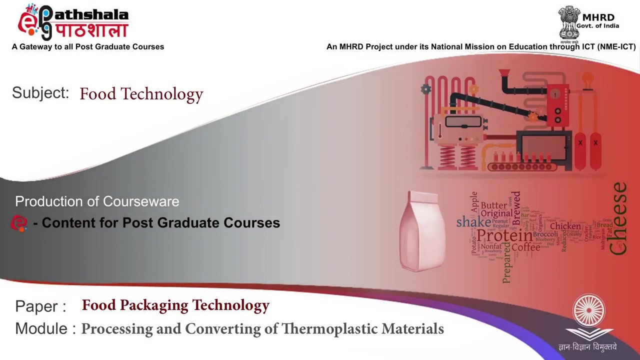 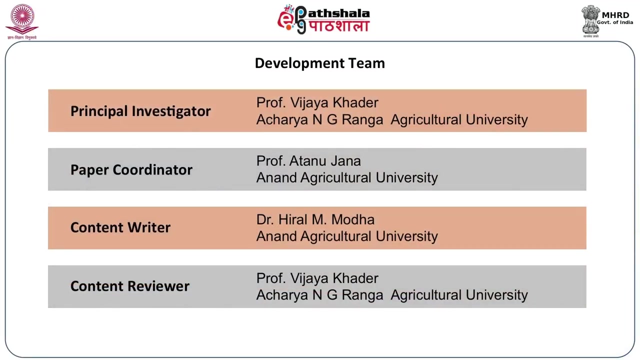 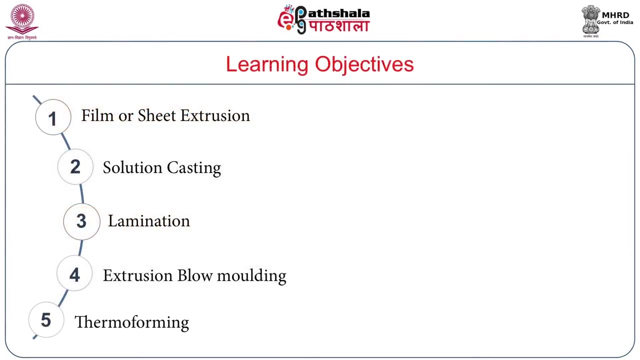 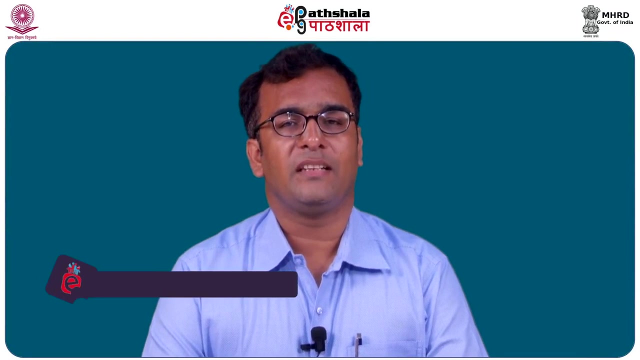 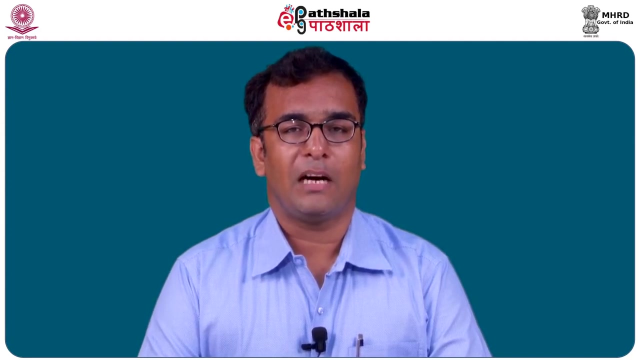 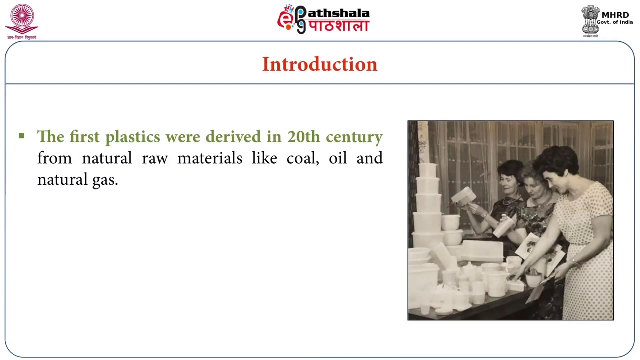 Hello friends, welcome back to our channel. In this module we will learn about different plastics and the formation techniques or different forms of packages can be formed, how they can be formed and what are the methods used for forming of different plastic forms. The first plastics were delivered in 20th century from natural raw materials like coal, oil and natural gas. 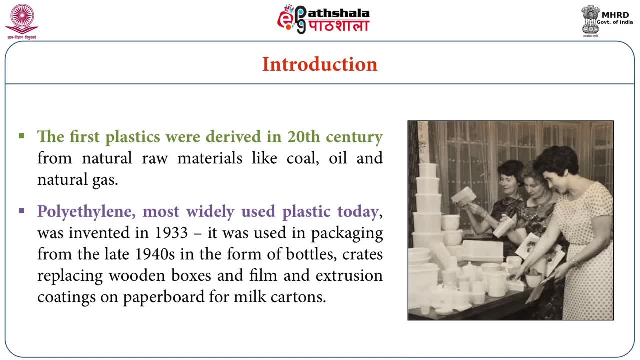 Polyethylene, most widely used plastic today, was invented in 1933. It was used in packaging from the late 1940s in the form of bottles, crate replacing wooden boxes, and film and extrusion coatings on paper board for milk cartons. 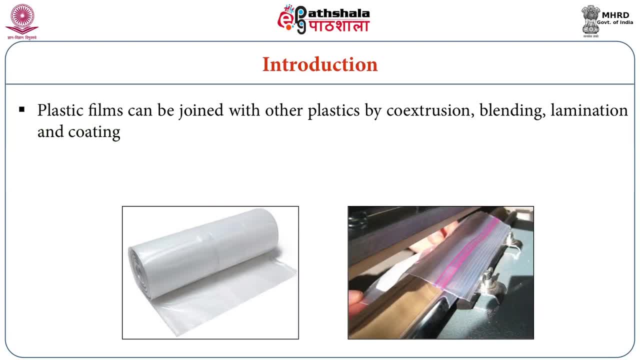 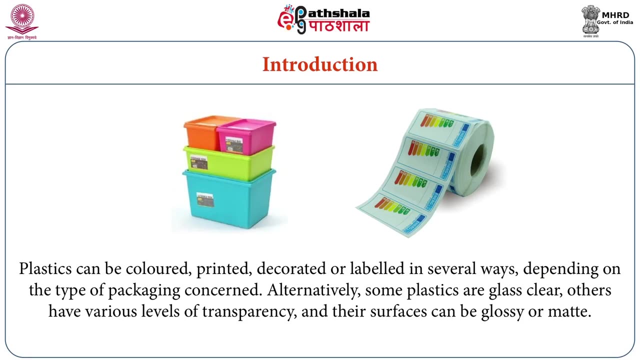 Plastic films can be joined with other plastics by co-extrusion, blending, lamination and coating to get properties which are components Plastic products could not provide alone. Plastics can be colored, printed, decorated or labeled in several ways, Depending on the type of packaging concerned. alternatively, some plastics are glass clear, others have various levels of transparency, and their surfaces can be glossy or have matte finish. 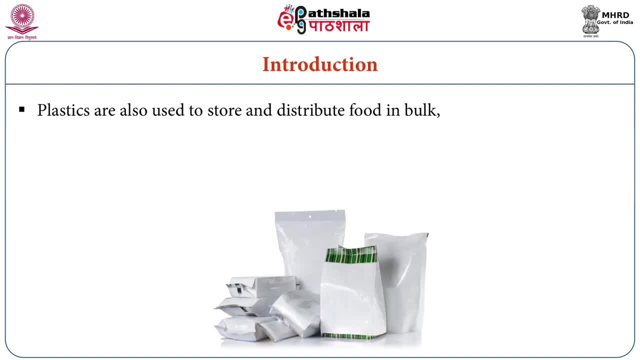 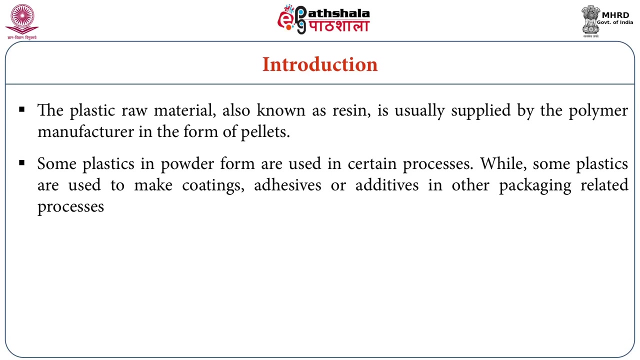 Plastics are also used to store and distribute food in bulk in form of drums. They can be stored for companies cheaper and Euro, who vacuum packs, zaps or ice packs. Linookaρο plastics contain 0.. solution for electrical source material in many processes. 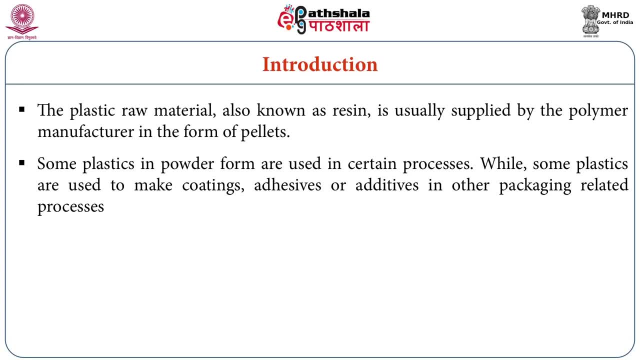 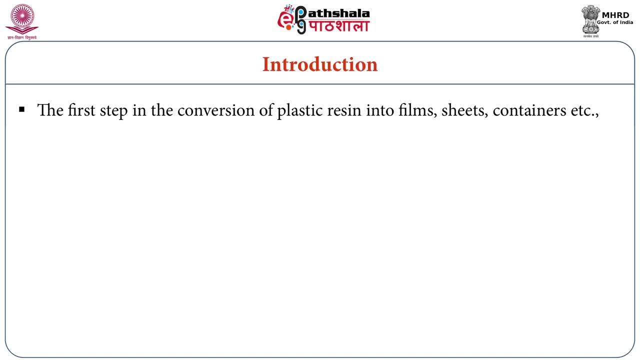 It has a composting power of up to 11 % its yield. xuo的話a xset in the form of air in other packaging related processes. The first step in the conversion of plastic resin into film sheets, containers etc. is to change the pellets from solids to liquid. 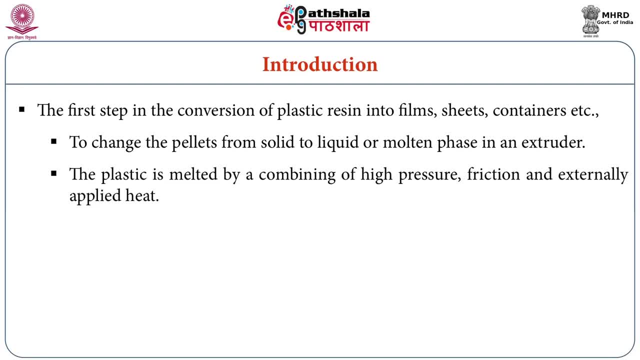 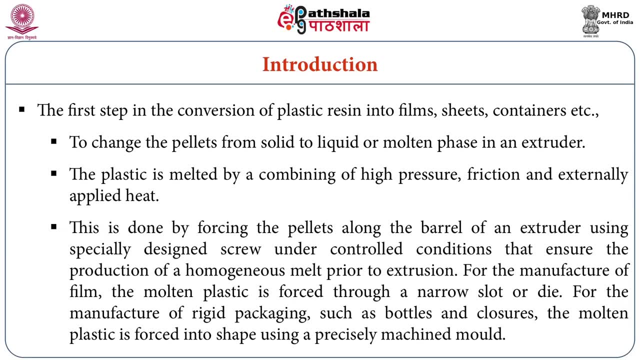 or molten phase in an extruder. The plastic is melted by combining of high pressure, friction and externally applied heat. This is done by forcing the pellets along the barrel of an extruder using specially designed screw under controlled conditions that ensure that production of a homogeneous melt prior to extrusion. 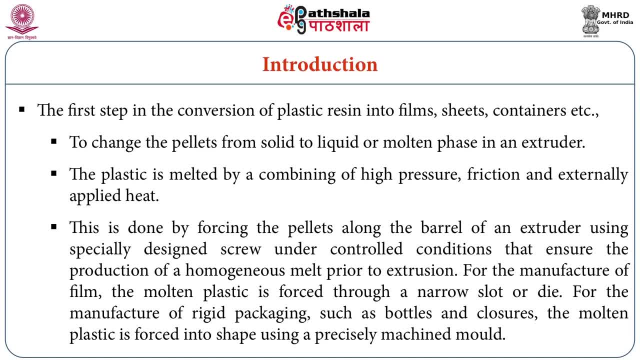 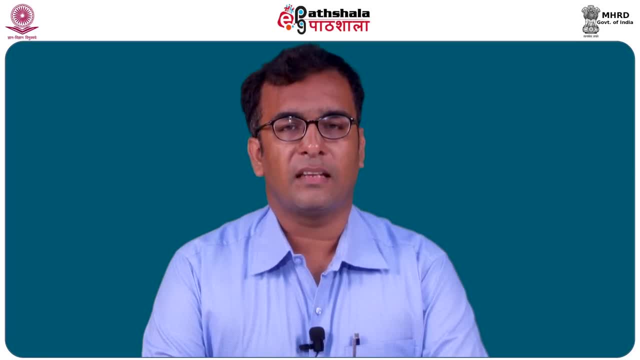 For the manufacture of film, the molten plastic is forced through a narrow slot or die. For the manufacture of packaging, such as bottles and closers, the molten plastic is forced into shape using a precisely machined mould. In this slide we 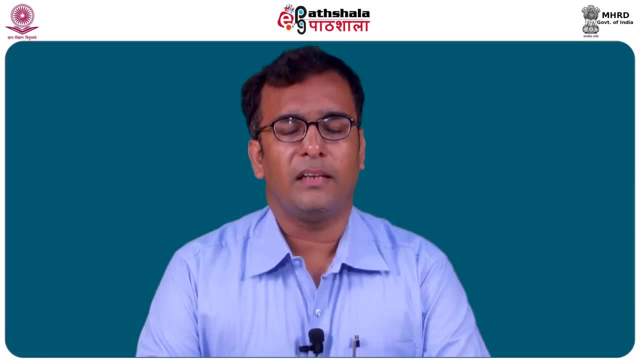 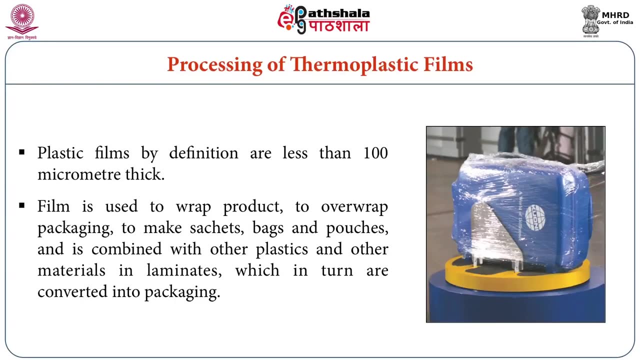 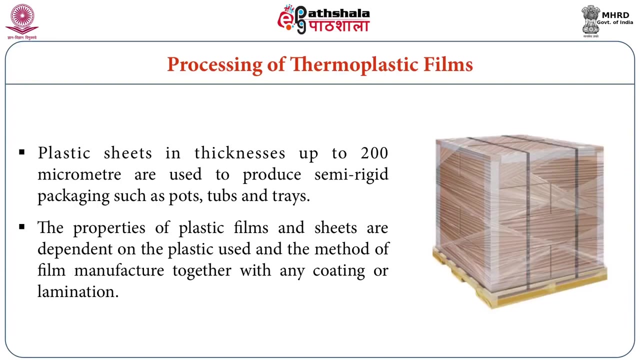 will learn about different plastic films. The films are normally having thickness below 100 microns and they are used for packaging of different food material as overwrap or can be formed into sachets or bags, etcetera, While the plastic sheets are having thickness. 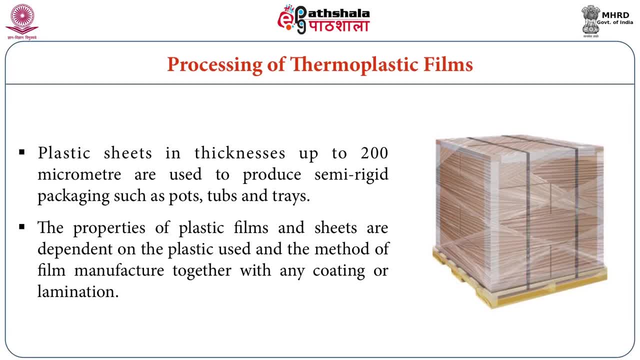 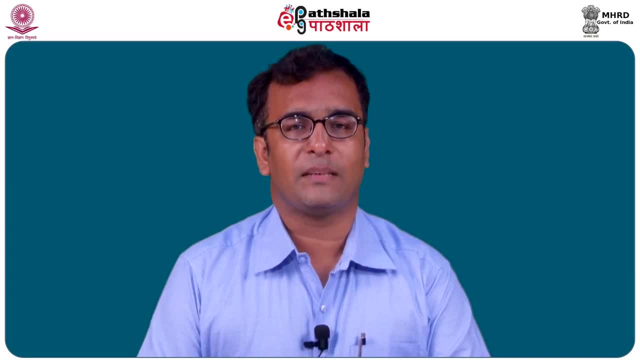 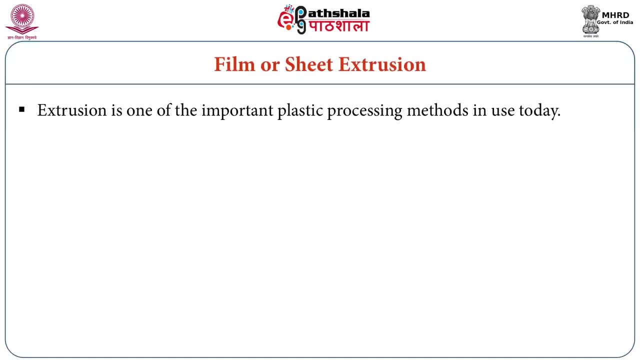 up to 200 microns, and they can be converted into different pots, cups, tubs, etcetera. The properties of film or the sheet depends on the type of plastic material used, as well as the different laminations has been carried out. Film and sheet extrusion. Extrusion is of the important plastic processing methods used. 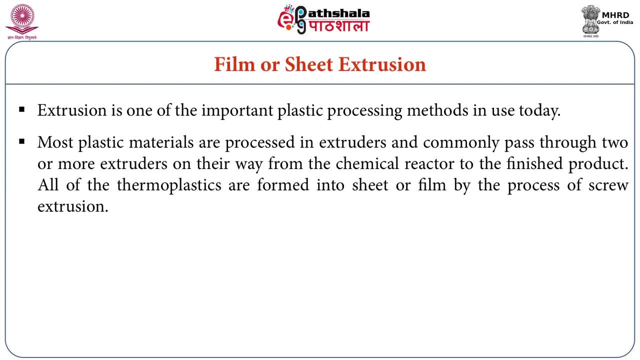 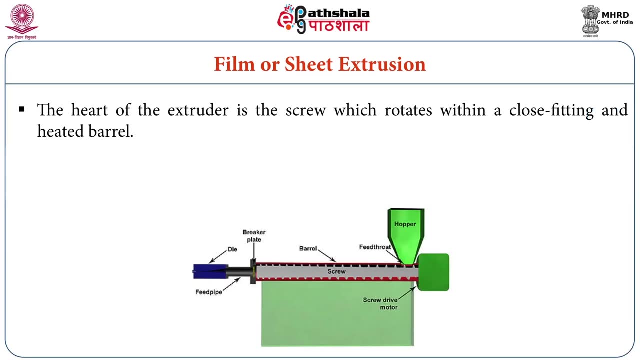 today, Most plastic materials are processed in extruders and commonly pass through two or more extruders on their way from chemical reactor to the finished product. All of the thermoplastics are formed into sheet or film By process of screw extrusion. the heat of extruder is the screw which rotates within. 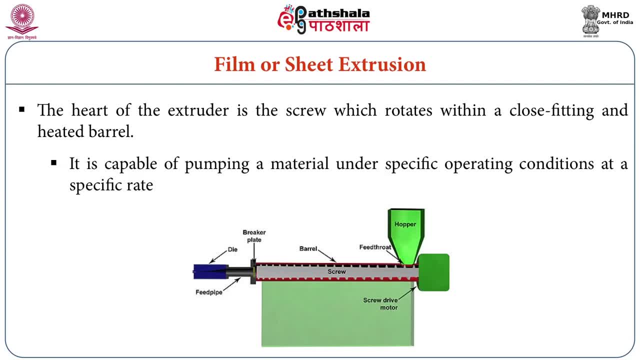 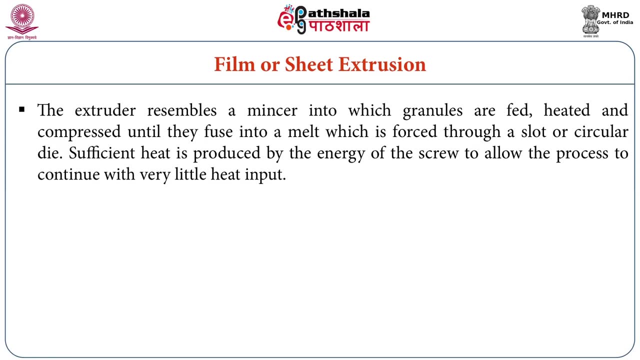 close fitting and heated barrel. It is capable of pumping a material under specific operating conditions, at a specific rate, depending on the resistance at the delivery and against which the extruder is required to pump. The extruder resembles a mincer into which granular 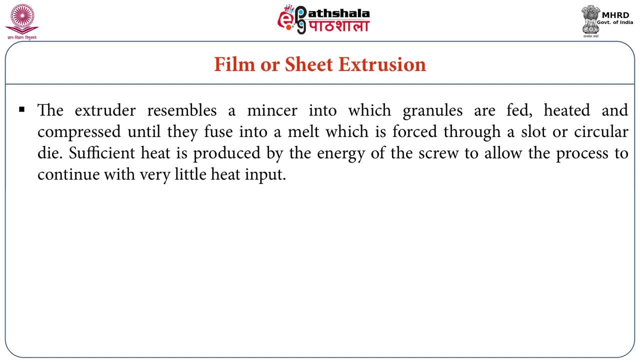 particles are fed, heated and compressed until they fuse into melt, which is forced through a slot or circular die. Sufficient heat is produced by the energy of the screw to allow the process to continue with very little heat input. There are basically two processes by which the extruded thermoplastic can be converted into film: The tubular process. 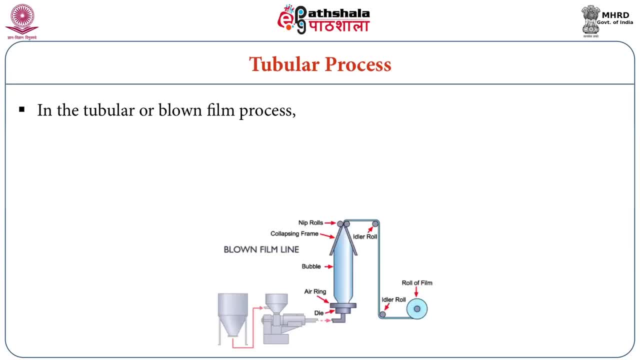 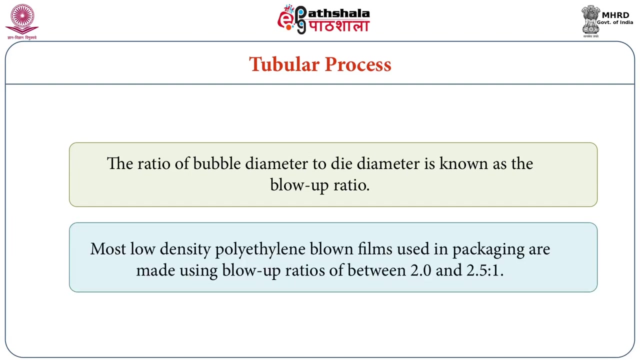 and the flat film process, The tubular process, A thin tube is extruded and by blowing air through the die head, the tube is inflated into a thin bubble which is cooled, flattened out and wound up. The ratio of bubble diameter to die diameter is known as blow-up ratio. Most low density polyethylene blown films. 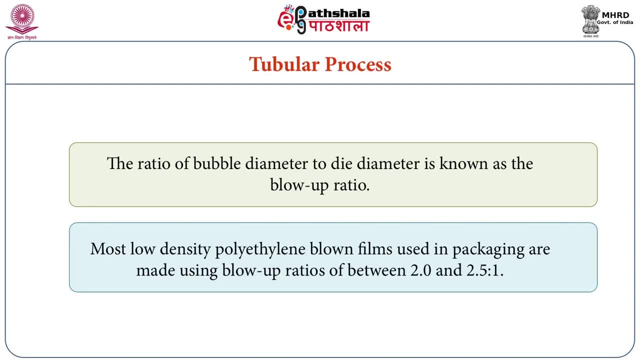 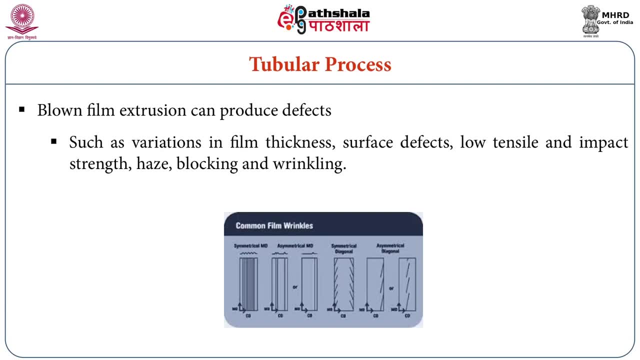 used in packaging are made using blow-up ratios of 2 to 2.5 is to 1.. Blown film extrusion can produce defects, such as variations in film thickness, surface defects, low tensile and impact strength, haze blocking and wrinkling. The properties of the film depend strongly. 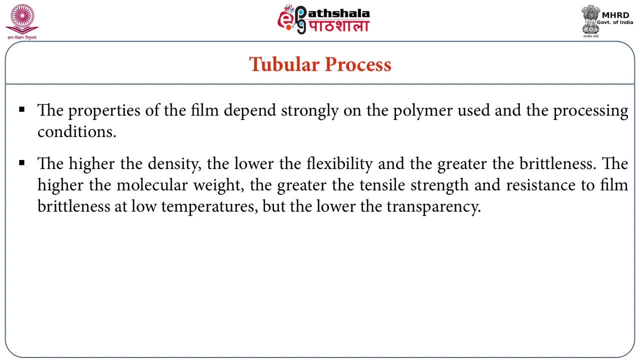 on the polymer used and processing conditions. The higher the density, the lower the flexibility and greater the brittleness. The higher the molecular weight, the greater the tensile strength and resistance to film brittleness at low temperatures, But the lower the transparency. 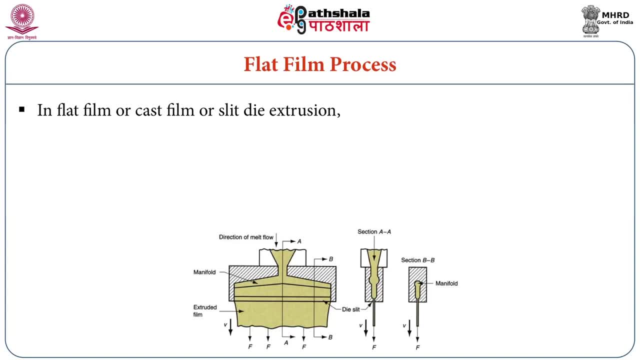 the higher the typhoon10 and höher the brand density. Another method is a flat film process. It is also known as cast-film or slate-dye-extrusion. The molten polymer is extruded through a slate-dye into a quenching bath or on to a chilled roller. 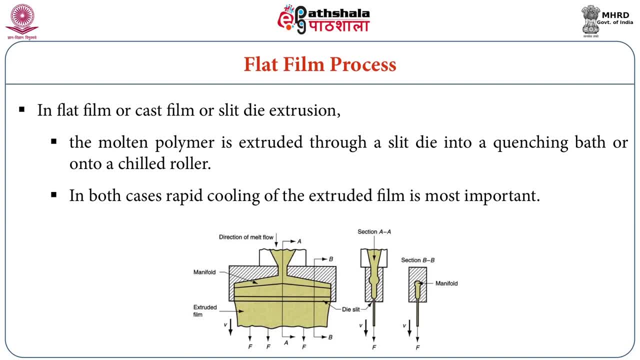 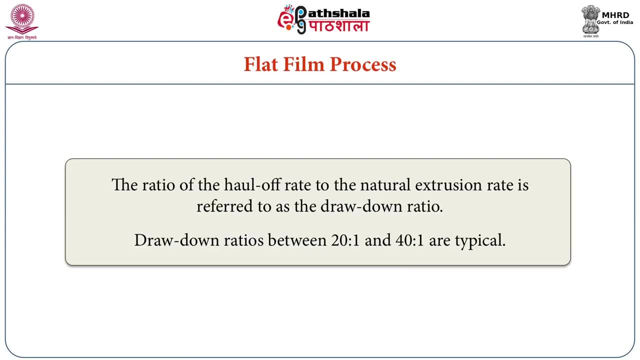 In both cases, rapid cooling of the extruded film is most important. The ratio of hol successor to the natural extrusion rate is referred to as draw down ratio. Draw down ratios between 1 to 40 is to 1 are generally typical. The advantages of flat film processes include: 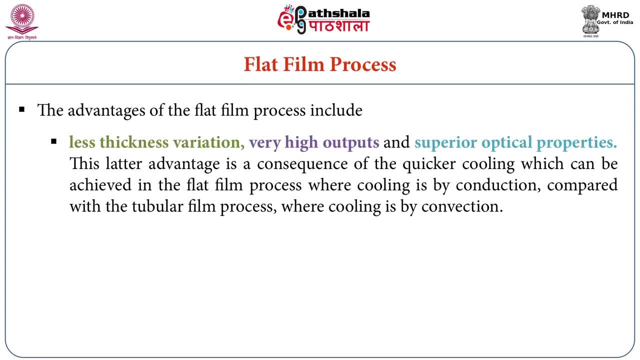 less thickness, variation, very high outputs and superior optical properties. This later advantage is consequence of the quicker cooling which can be achieved in the flat film process, where cooling is by conduction, compared with the tubular film process, where cooling is done by convection. 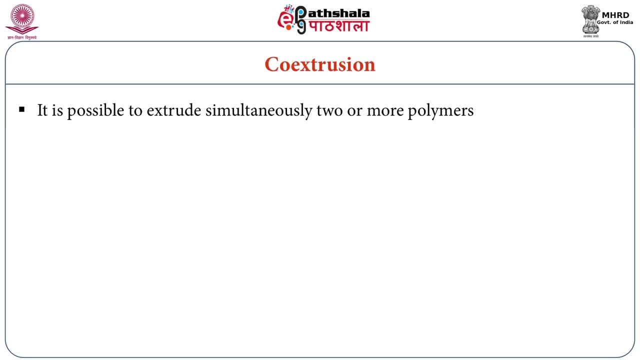 Next process is co-extrusion. It is possible to co-extrude simultaneously two or more polymers which fuse at the point of film formation into a single web by using combination adapters. Such process is known as co-extrusion and permits the production of single web having. 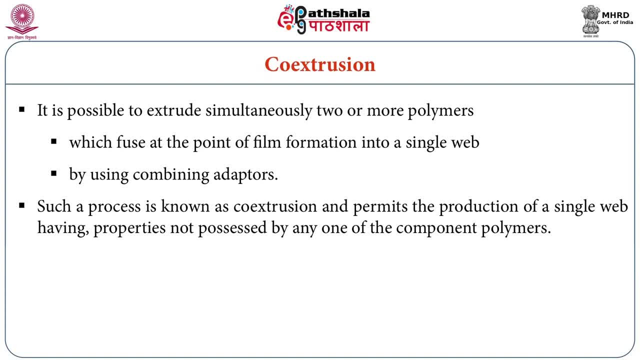 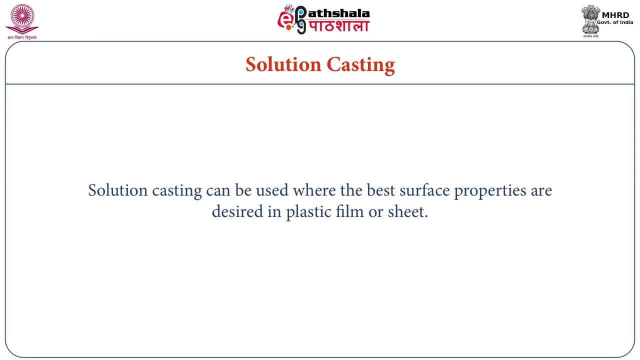 properties not possessed by any one of the component polymers. A two component slot die is capable of producing a two or three layer film, While a three component die can produce a five layer film from three materials. Next method is solution casting. It can be used where the best surface properties are. 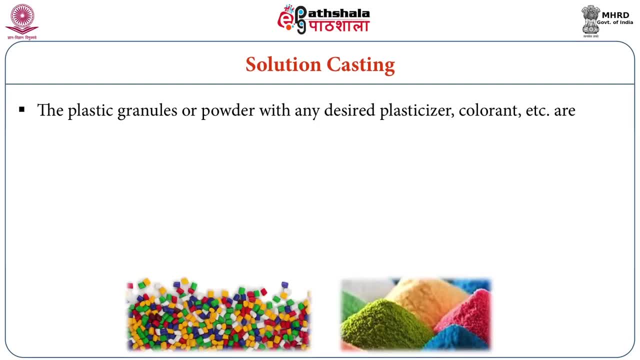 desired in plastic, film or sheet. The plastic granules or powder with any desired plasticizer, colorant etc. are dissolved in a suitable solvent. After filtering, the solution is cast from a slot die onto a moving highly polished stainless steel belt. The solvent. 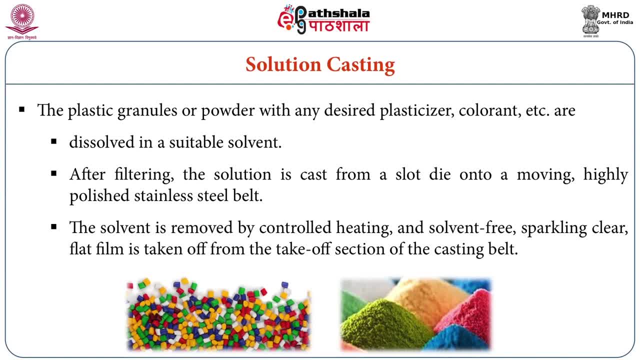 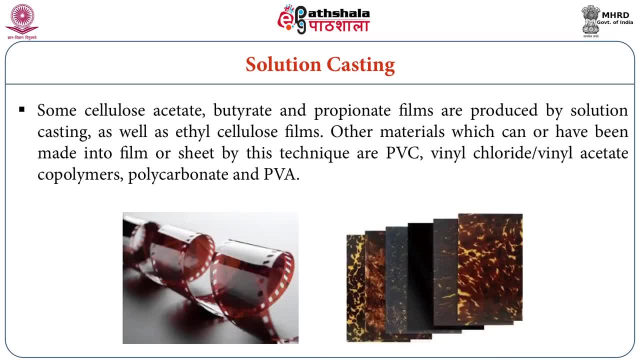 is removed by controlled heating and solvent free. sparkling clear, flat film is taken off from take off section of the casting belt. Some cellulose acetate, butyrate and propionate films are produced by solution casting, as well as ethyl cellulose films, Other materials which can or have been made into film or sheet. 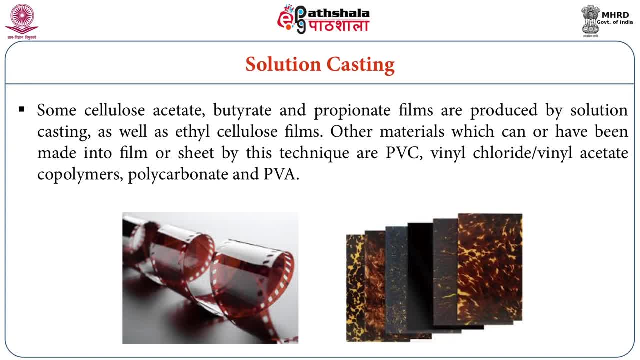 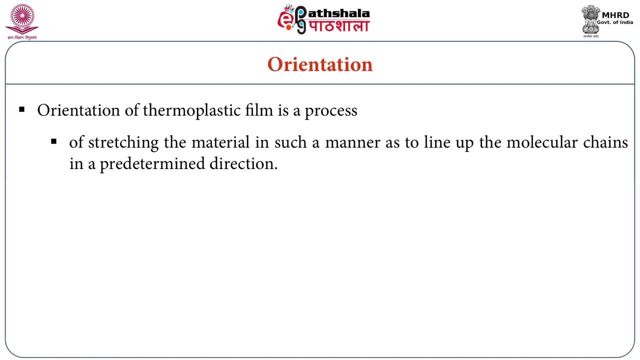 by this technique are PVC, vinyl chloride, vinyl acetate, copolymers, polycarbonate and PVA. Orientation of thermoplastic film is a process of stretching the material in such a manner as to line up the molecular chains in a predetermined direction. Once lined up the ordered arrangement: 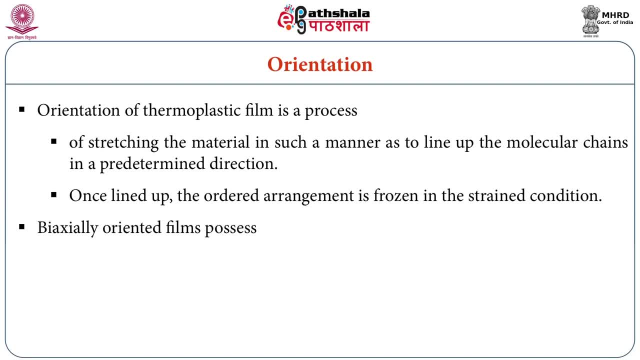 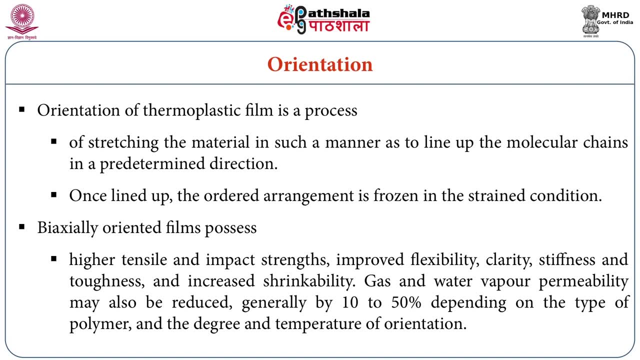 is frozen in the strained condition By actually oriented film possesses higher tensile and impact strength, improved flexibility, clarity, stiffness and toughness, and increased shrinkability. Gas and water vapor permeability may also be reduced, Generally by 10 to 50%, depending on the type of polymer and the degree and temperature. 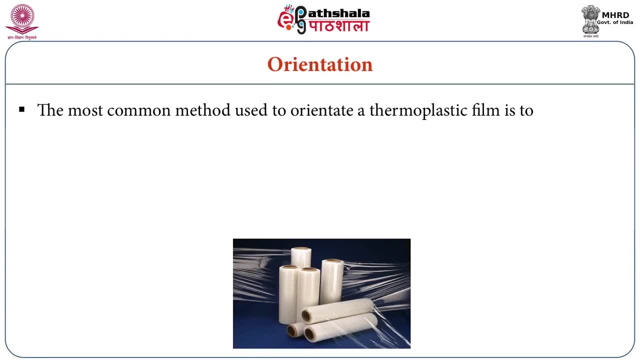 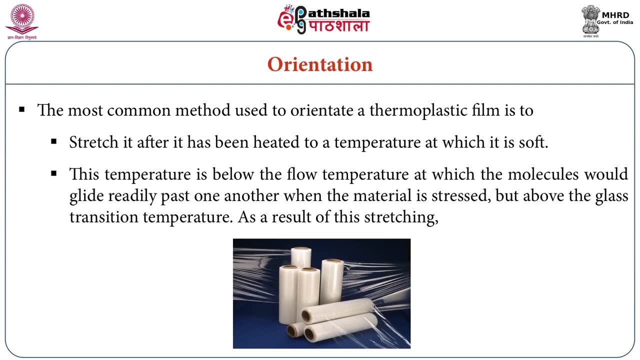 of orientation. The most common method used to orient a thermoplastic film is to stretch it, after it has been heated, to temperature at which it is soft. This temperature is below the flow temperature at which the molecules would glide readily past one another when the material is stretched, but above 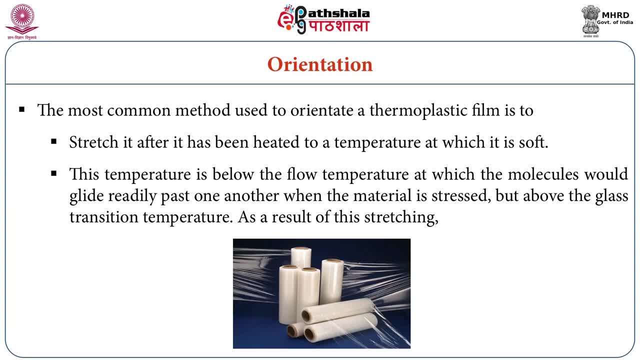 the glass transition temperature. As a result of this, the temperature of the film is reduced. The temperature of the film is reduced by 10 to 50 percent, depending on the type of polymer and the degree and temperature of the film. As a result of this stretching, the direction of the molecules changes towards that in which 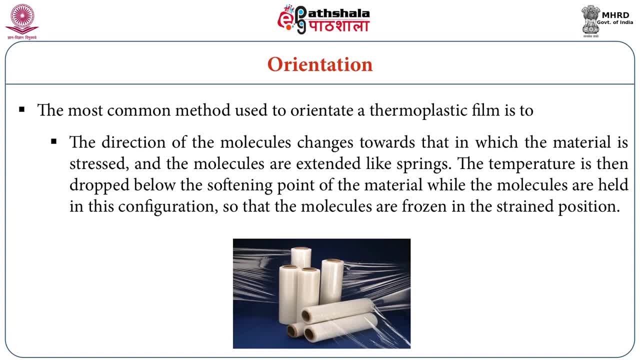 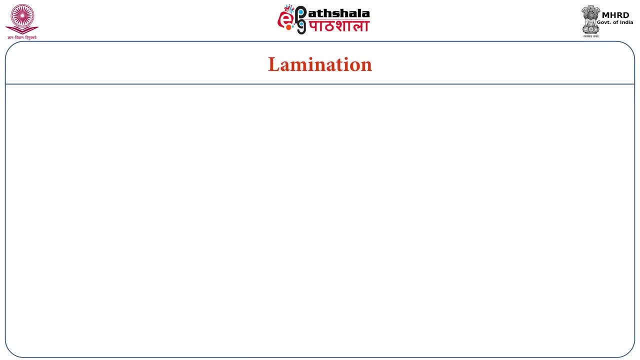 the material is stretched and the molecules are extended like springs. The temperature is then dropped below the softening point of the material, while the molecules are held in this configuration, so that the molecules are frozen in the strained position, which improves the properties. Next method is lamination, Although lamination is the process of bringing two or more webs. 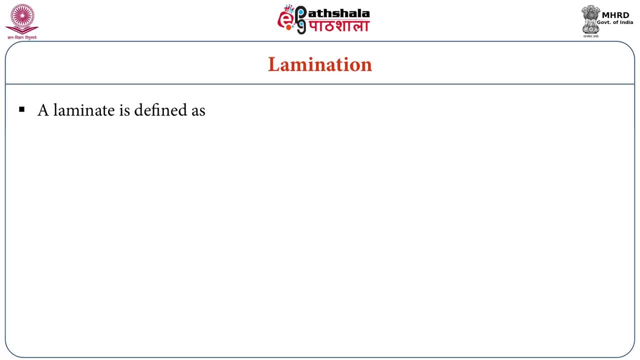 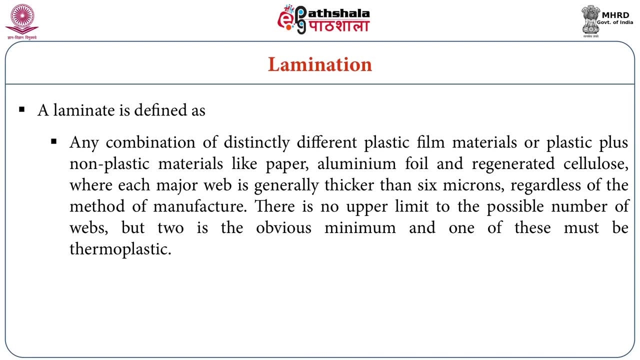 together and bonding them with an adhesive or by heating. a laminate is defined as any combination of distinctly different plastic film materials or plastic plus non-plastic materials like paper, aluminum foil and regenerated cellulose, where each major web is generally thicker than six microns, regardless of the method of manufacture. 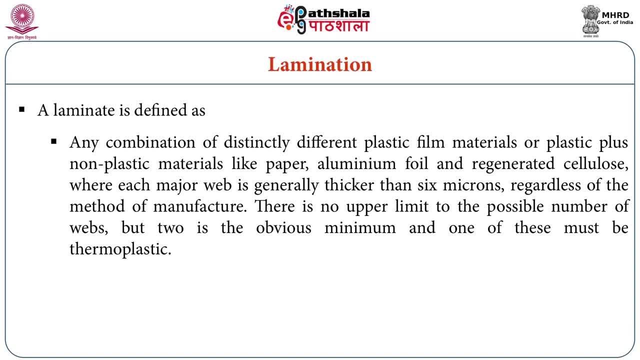 There is no upper limit to the possible number of webs, but two is the obvious minimum, and one of this must be thermoplastic, And in the case of a laminated plastic, the thickness of the material used should be equal to the thickness of the material. Well, since the plastic 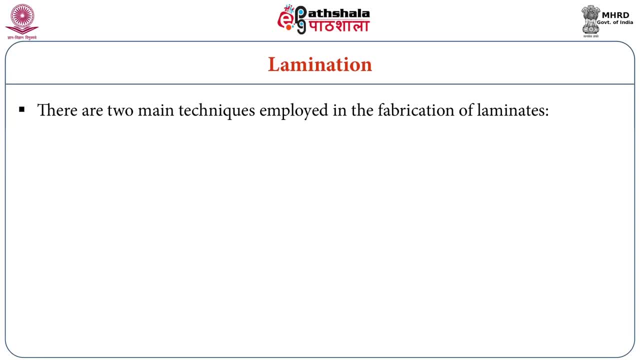 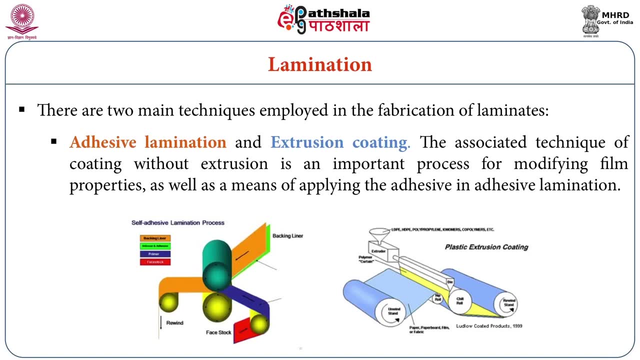 There are two main techniques employed in the fabrication of laminates: adhesive lamination and extrusion coating. The associated techniques of coating without extrusion is an important process for modifying film properties, as well as a means of applying the adhesive in the adhesive lamination. 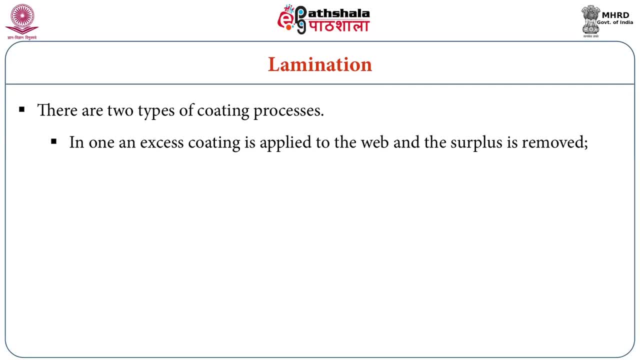 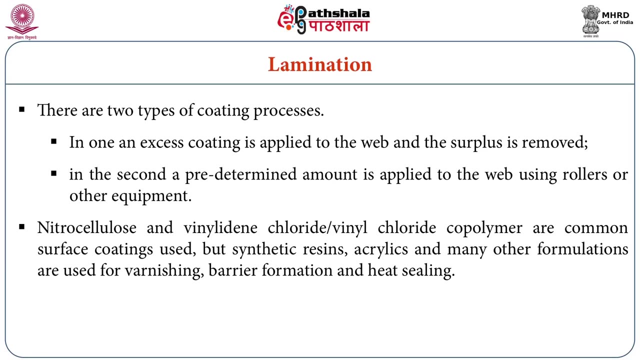 There are two types of coating processes. In one, an excess coating is applied to the web and the surplus is removed. In the second, a predetermined amount is applied to the web using rollers or other equipment. Nitrocellulose and vinylidene chloride- vinyl chloride copolymers are common surface coatings. 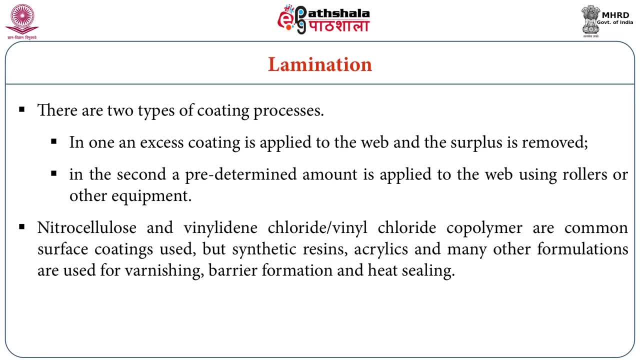 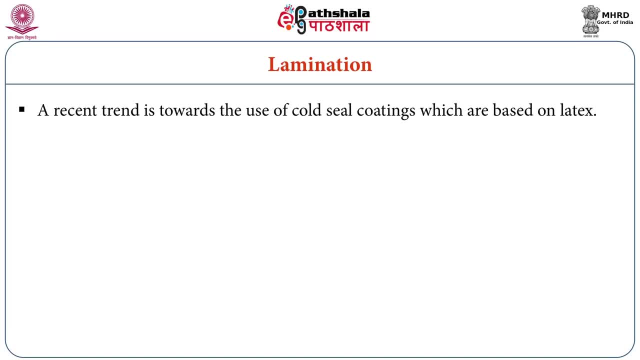 used, but synthetic resins, acrylics and many other formulations are also used for varnishing, barrier formation and heat sealing. A recent trend is towards the use of cold seal coatings, which are based on latex. They require only contact pressure If a particular coating does not arrive on the surface before the job is completed, it. 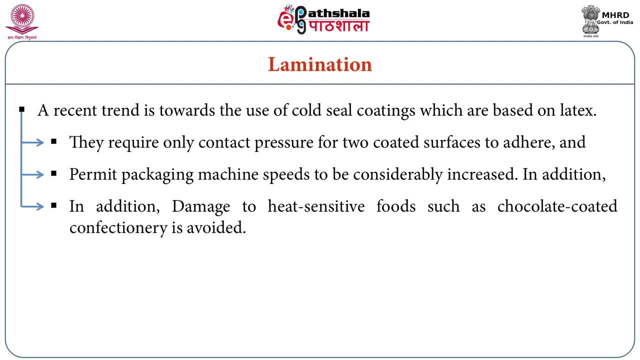 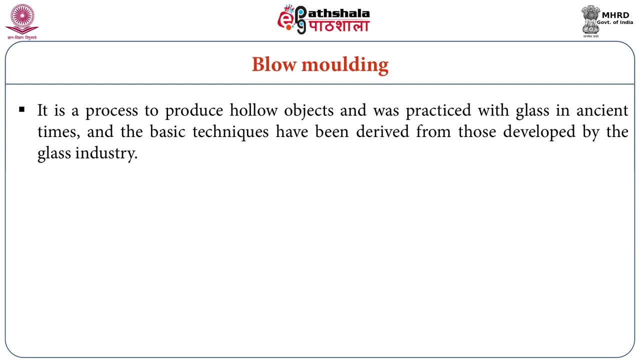 may be difficult to remove it. The other type of coatings are a box molding, which is used for the application of a plastic coating to a mold. This is equivalent to the application of a rubber roller to a metal plate to made the mould. It is called a box molding and is the type of molding that is used to create uncoated. 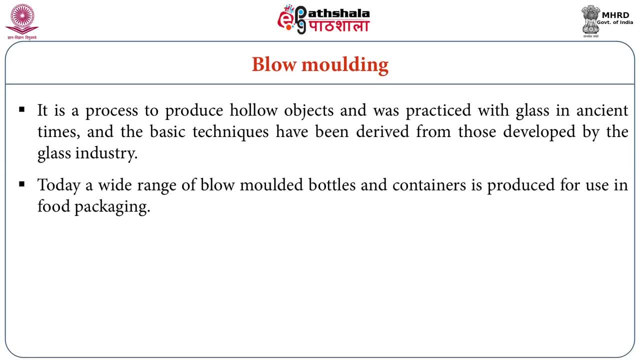 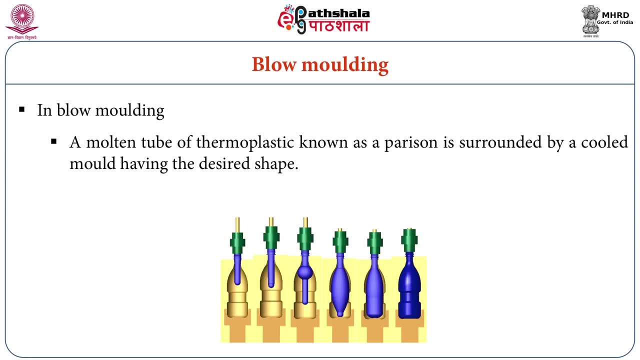 paper, paper. This is the type of molding that can be used to create a box molding. It requires a thin press ball. It is a thin press ball produced for use in food packaging In blow molding, a molten tube of thermoplastic known. 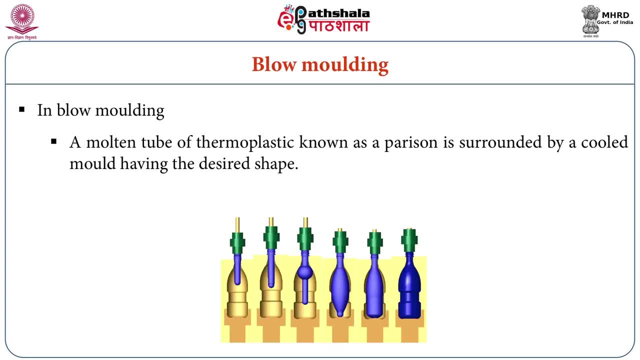 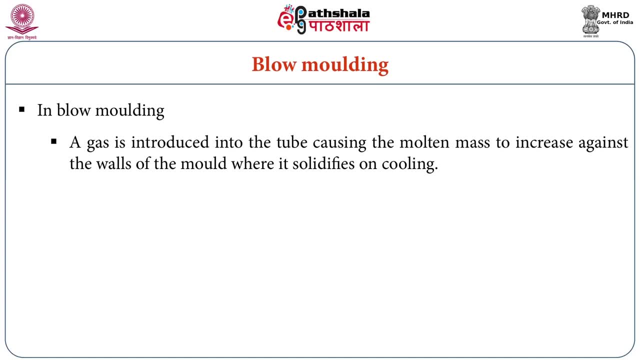 as parison, is surrounded by a cooled mold having the desired shape, A gas is introduced into the tube, causing the molten mass to increase against the wall of mold, where it solidifies on cooling. The mold is then opened and the bottle is ejected. Normally, the process consists of: 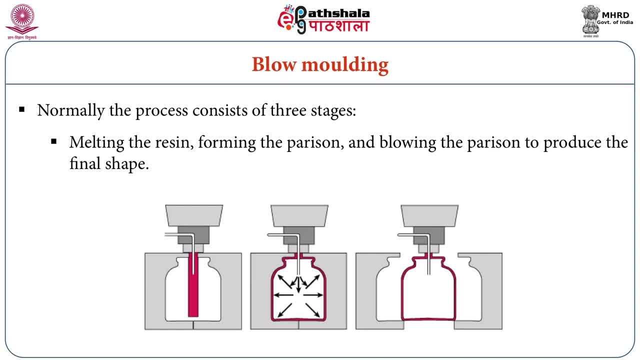 three stages: melting the resin, forming the parison and blowing the parison to produce the final shape. The blowing step may take from a few seconds to more than a minute for large shapes. The rate limiting step is cooling of the molded shapes. There are two techniques for plasticizing. 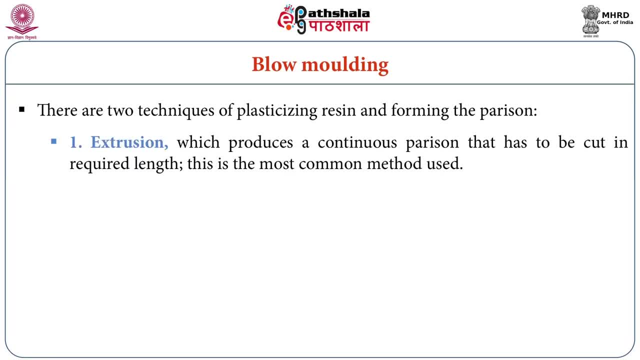 resin and forming parison Extrusion, which produces a continuous parison that has to be cut into required length. This is the most common method used. Another one is injection molding, where the parison is formed in one mold and then transferred into another mold for blowing Extrusion. blow molding: 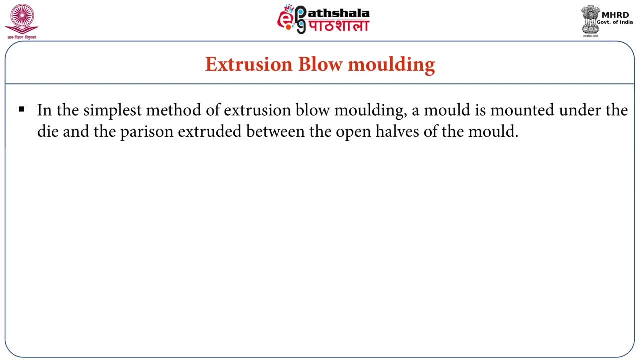 In the simplest method of extrusion blow molding, a mold is mounted under the die and the parison extruded between the open halves of the mold. When the parison reaches the proper length, the extruder is stopped and the mold closes around the parison. 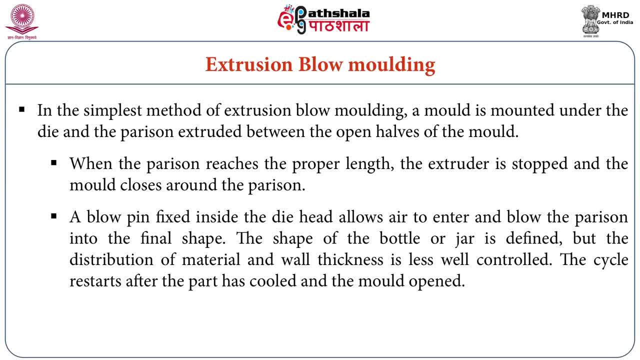 The blow pin fixed inside the die head allows air to enter, the blow the parison into final shape. The shape of bottle or jar is defined, but the distribution of material and wall thickness is less well controlled. The cycle restarts after the part has cooled and the mold opened. 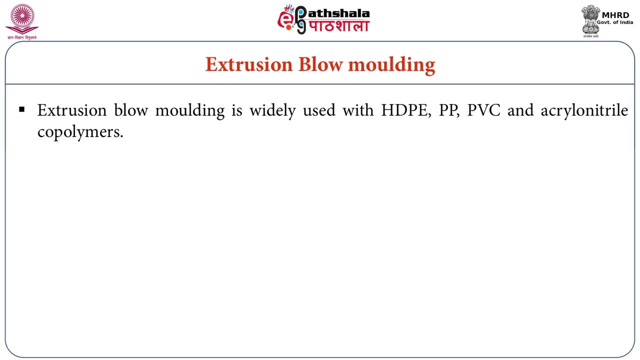 Extrusion blow molding is widely used with HDPE, PP, PVC and acrylonitrile copolymers. Common grades of PET cannot be extrusion blown. A development in the production of co-extruded bottles where two or more extruders each. 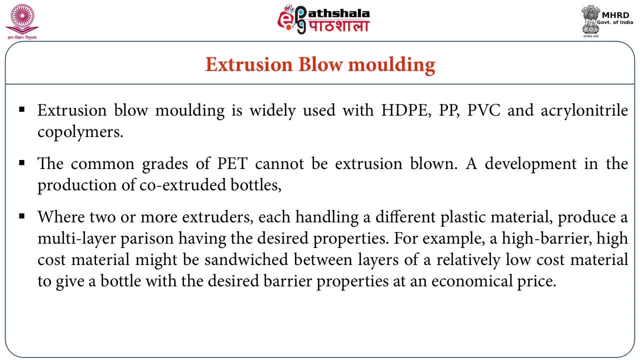 handling a different plastic material, produce a multi-layered parison having the desired properties. For example, a high-barrier, high-cost material might be sandwiched between layers of relatively low-cost material to give a bottle with the desired barrier properties as an economical price. 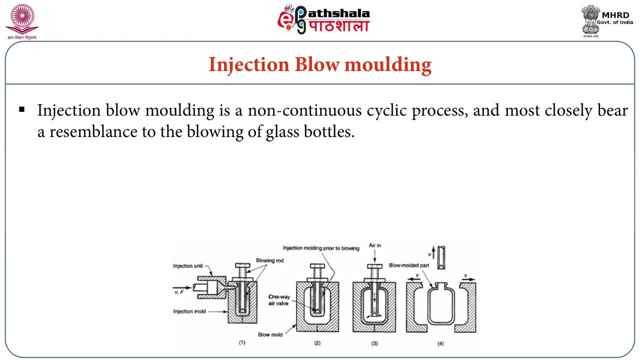 Ex. Another method is injection blow molding. It is a non-continuous, cyclic process and most closely bear resemblance to blowing of glass bottles. The parison is formed in one mold and then, while still molten, is transferred to a second mold, where blowing with compressed 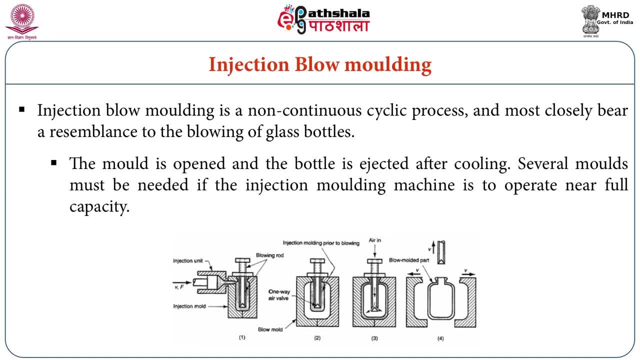 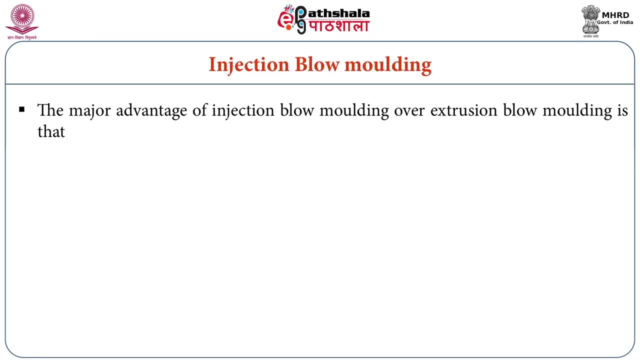 air forms the final shape, The mold is opened and the bottle is ejected after cooling. Several molds must be needed if the injection molding machine is to operate near full capacity. The major advantage of injection blow molding over extrusion blow molding is that the process 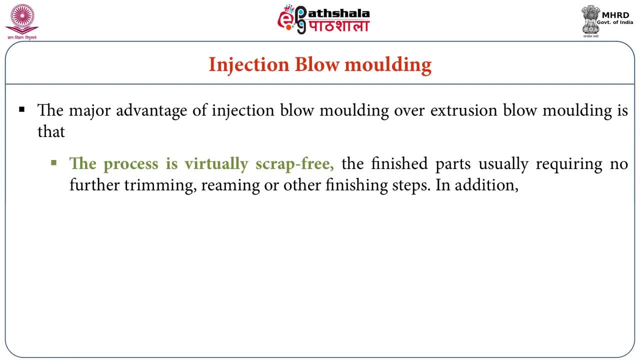 is virtually scrap-free, the finished part usually requiring no further trimming, reaming or other finishing steps. In addition, the dimensions of bottle show very slight variation from bottle to bottle and with some materials, improved strength and clarity are attained due to the effect of limited degree. 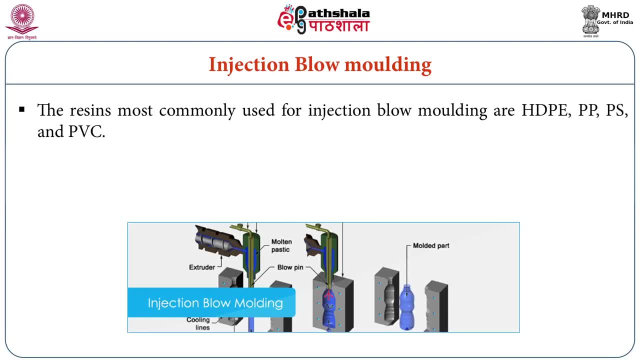 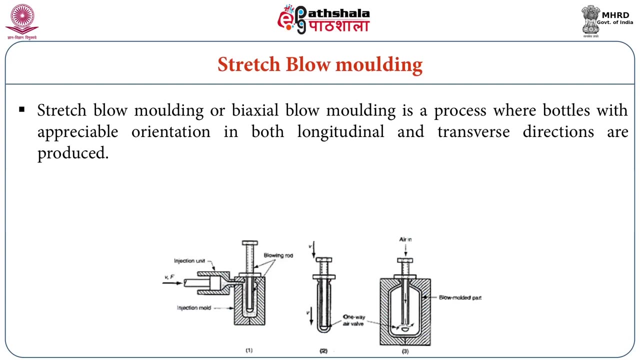 of biaxial orientation. The resins most commonly used for injection blow molding are HDP, PP, PS and PVC. Recently, PET has been injection blow molded and is likely to replace PVC in some applications. Stretch blow molding, or biaxial blow molding, is a process where bottles 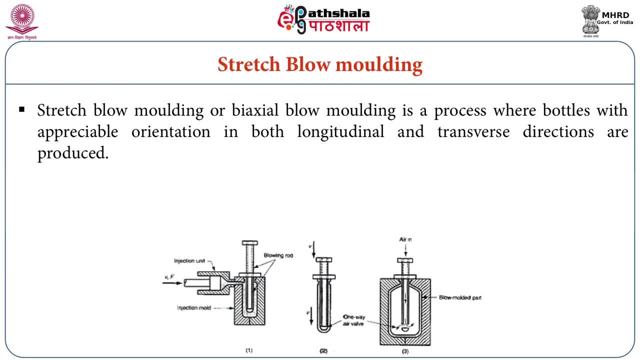 with appreciable orientation are removed from the bottle. The process of injection, blow molding and transfer orientation in both longitudinal and transfer direction are produced To produce a biaxially molded bottle. a parison is stretched longitudinally under heat and blown into bottle. 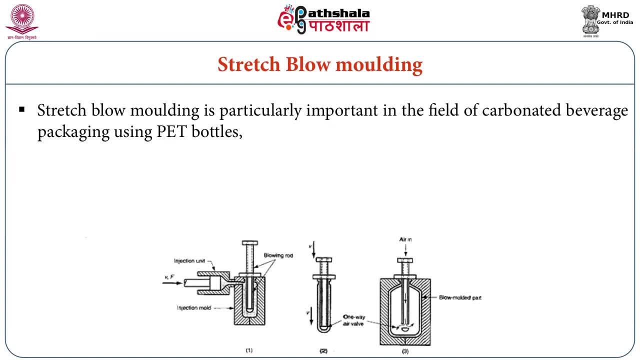 with consequent transfer orientation. Stretch blow molding is particularly important in the field of carbonated beverage packaging using PET bottles, but is limited to relatively simple bottle shapes. For best results, the resin molecules must be conditioned, stretched and oriented at just above the glass transition temperature. 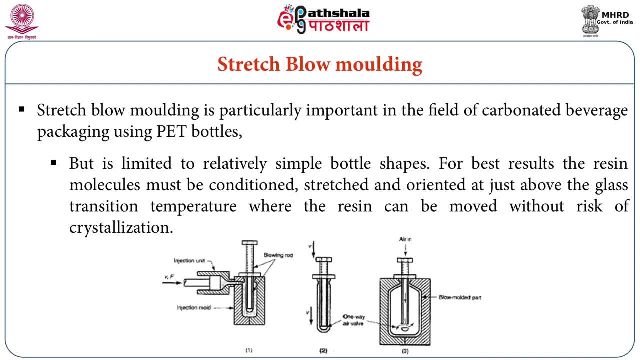 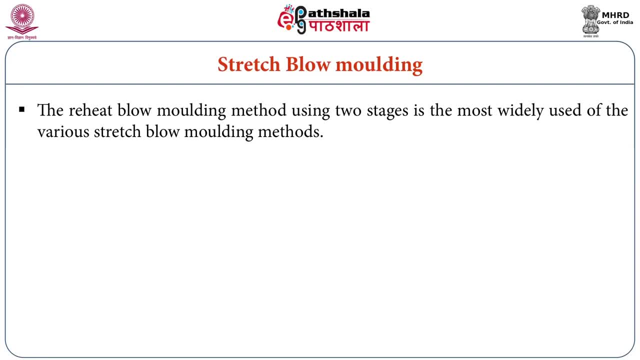 when the resin can be moved without risk of crystallization. The reheat blow molding method using two stages is the most widely used of the various stretch blow molding methods. First, the parison are injection molded in a completely separate stage and stored at ambient temperature until required. They are 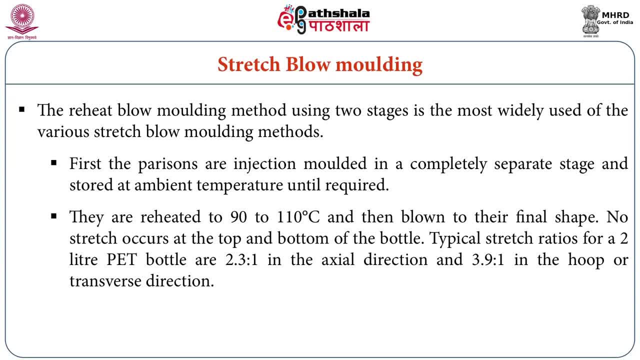 reheated to 90 to 110 degree centigrade and then blown to their final shape. No stretch color at the top and bottom of the bottle. The design is distinctly similar to that of the average Vega igen�니다. Typically stretch ratios for 2 litre PET bottles are 2.3x 1 in. 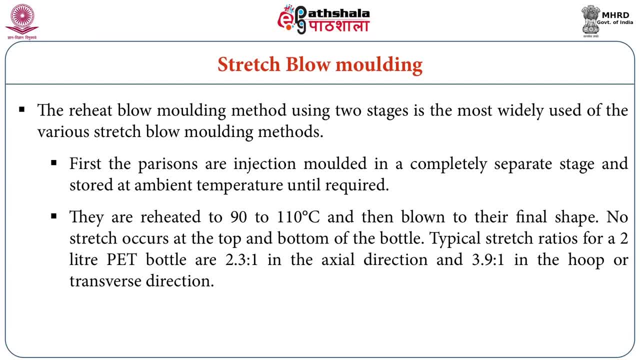 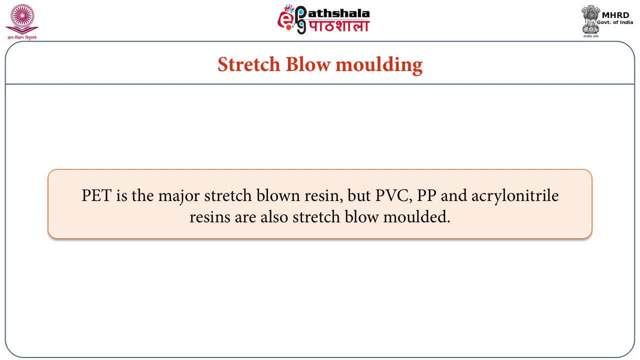 the axial direction and 3.9x. 1 in the hoop transverse direction. PET is the major stretch blown resinora, but PVC, PP, acrylic and vitalized resin, noble Baboon and Laurenum are also stretched blow molded along their possessed shape. Our specific��l sofas mosses contain two. 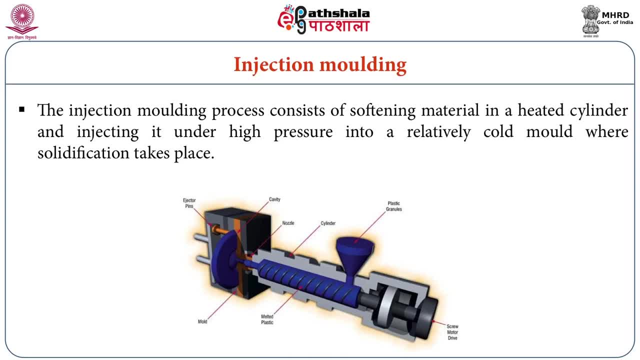 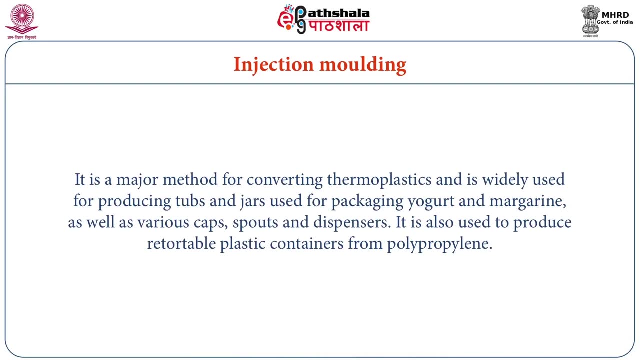 injection molding. This process is consists of softening material in a heated cylinder and injecting it under high pressure into a relatively cold mold where solidification takes place. It is major method for converting thermoplastics and is widely used for producing tubs and jars used for packaging yogurt and margarine, as well as various caps spouts. 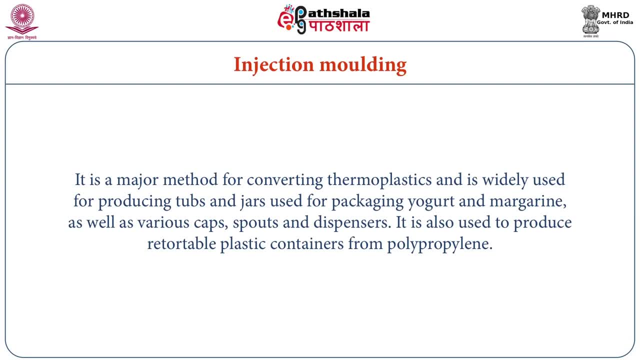 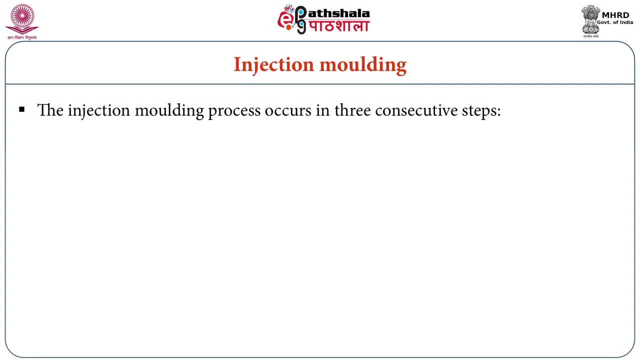 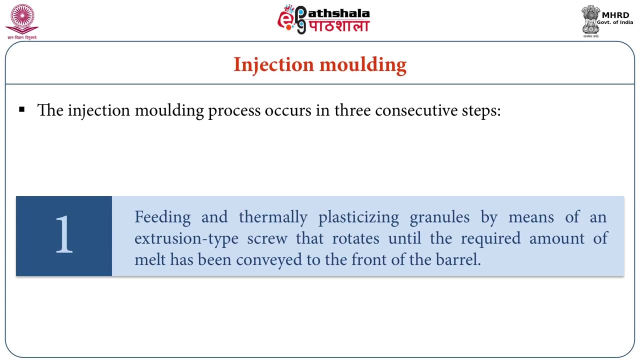 and dispensers. It is also used to produce retortable plastic containers from polypropylene. The injection molding process occurs in three consecutive steps. First one, feeding the thermally plasticizing granules by means of an extrusion type screw that rotates until the required. 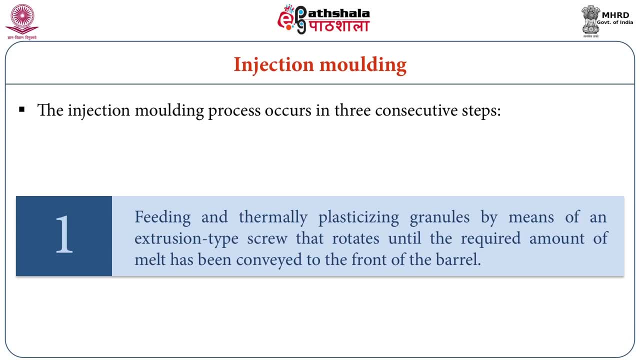 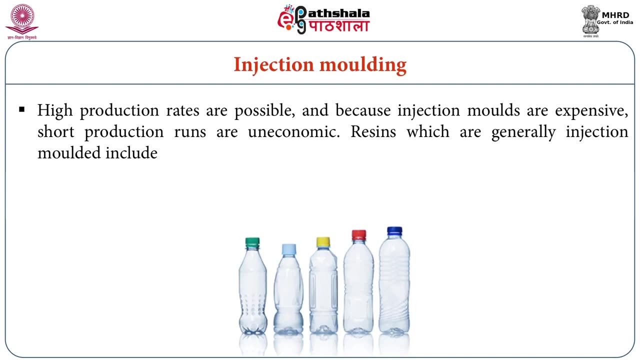 amount of melt has been conveyed to the front of the barrel. Second, injecting a calculated amount of stock into cold cavity. and third, cooling and ejecting the molded components. High production rates are possible and, because injection molds are expensive, short production runs are uneconomic. Resins, which are generally injection molded, include low and high density. 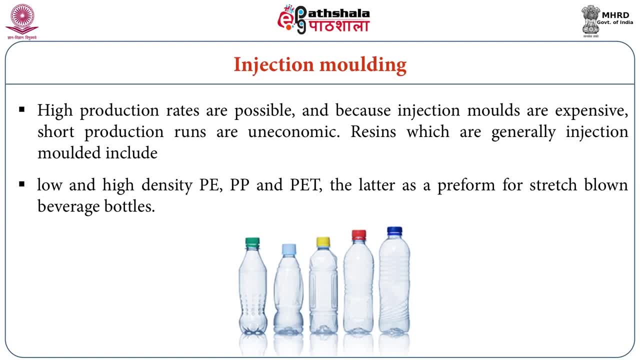 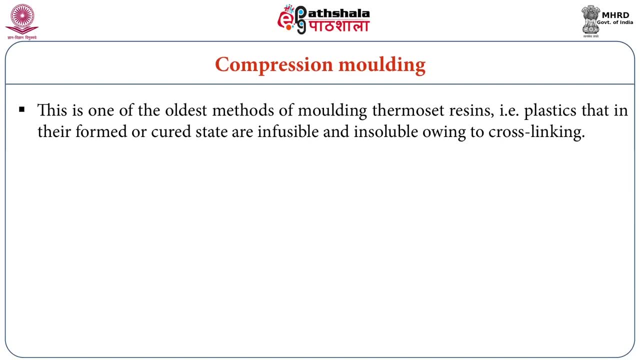 polyethylene, PP, PET, and the latter are preformed for stretch blown beverage bottles. Compression molding: this is one of the oldest method of molding thermoset resins, that is, plastics That, in their formed or cured state, are infusible and insoluble owing to cross linking It has. 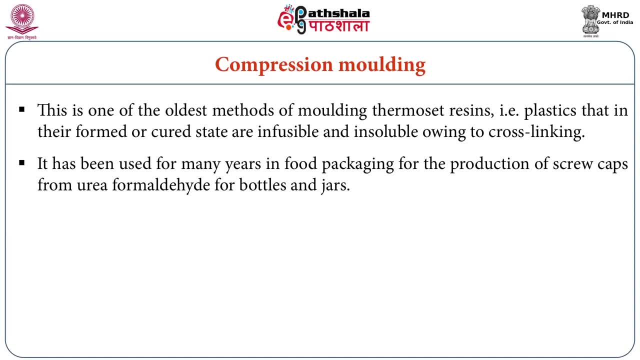 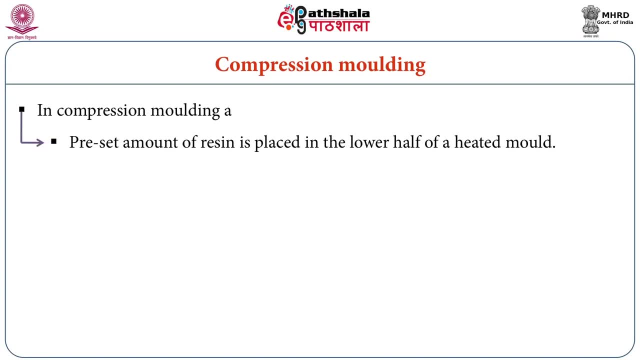 been used for many years in food packaging for the production of screw caps from urea formaldehyde for bottles and jars. Compression molding: a preset amount of resin is placed in the lower half of a heated mold. The top of the mold is then brought down into the 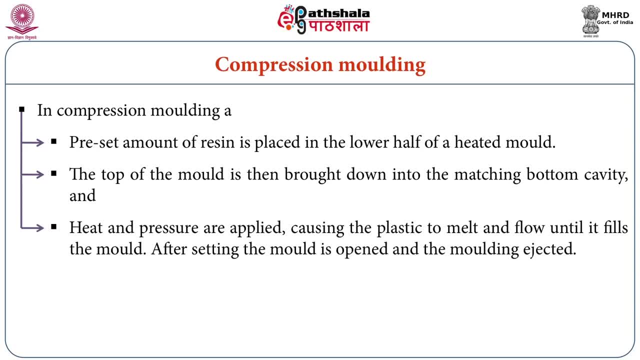 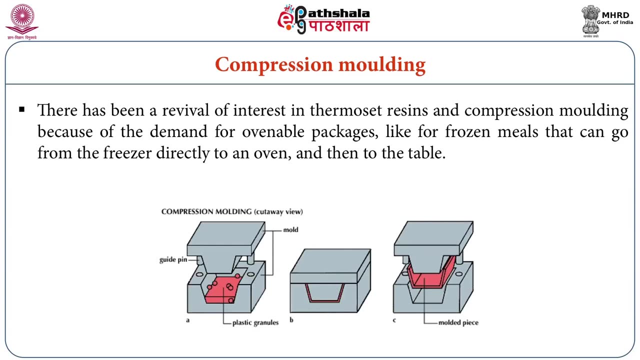 matching bottom cavity. So you can see the design of how molding is done. Now let's see the final product. So first let's see the process of plasticization of thermoset resin. There has been a revival of interest in thermoset resins and compression molding because of 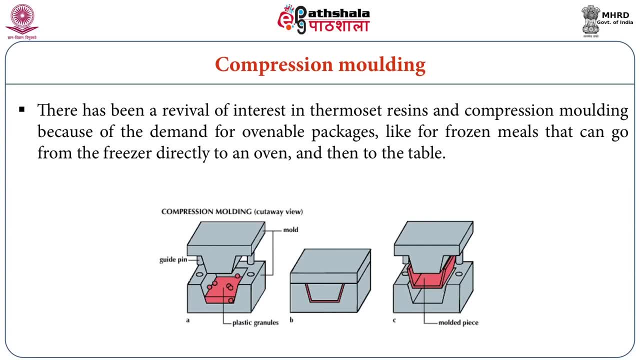 the demand for over-neuable packages, Like for frozen meals, that can go from the freezer directly to an oven and then to the table. But there are some interesting new elements to this process of molding, For example plastic molding, which we have seen is not completely frozen And which is on the setting of the 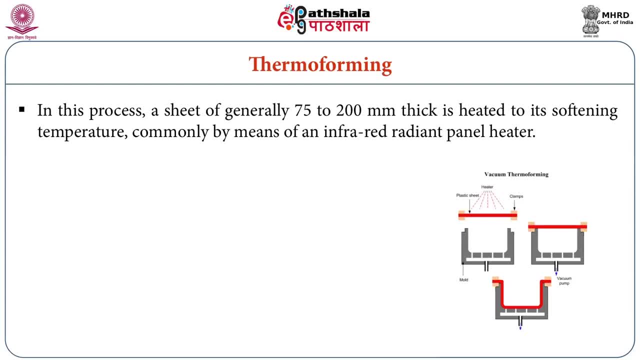 In this process, a sheet of generally 75 to 200 mm thick is heated to its softening temperature, commonly by means of an infrared radiant panel heater. By some pneumatic or mechanical means, the sheet is forced against a mold shape and, after cooling, the part is removed and trimmed. 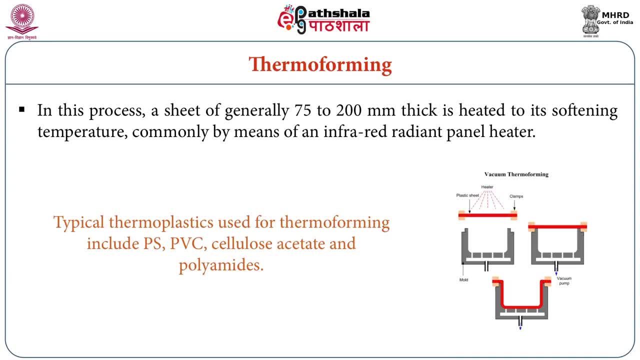 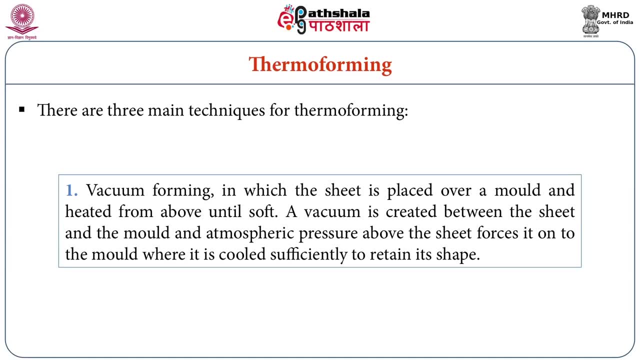 Typical thermoplastics used for thermoforming includes PS, PVC, cellulose acetate and polyamides. There are three main techniques for thermoforming. first is vacuum forming, in which the sheet is placed over a mold and heated from above until soft. 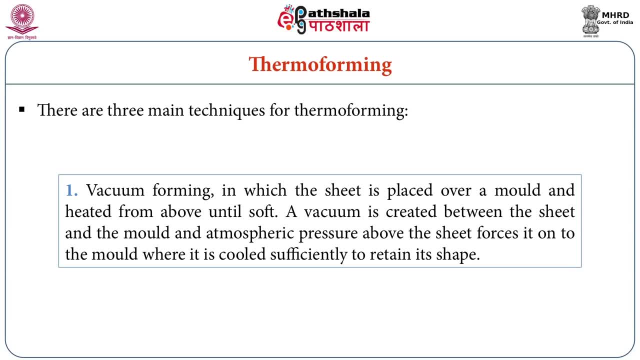 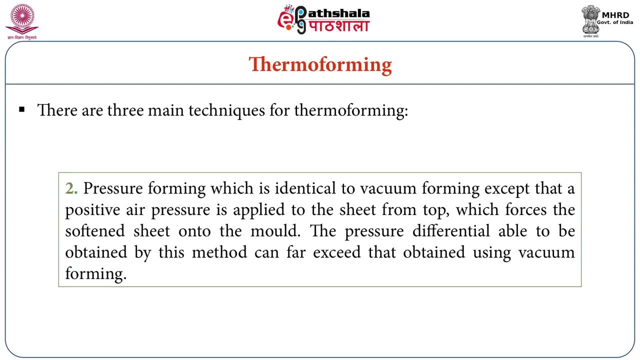 A vacuum is created between the sheet and the mold, and atmospheric pressure above the sheet forces it onto the mold, where it is cooled sufficiently to retain its shape. Second, one pressure forming, which is identical to vacuum forming, except that the positive pressure is applied to the sheet from top. 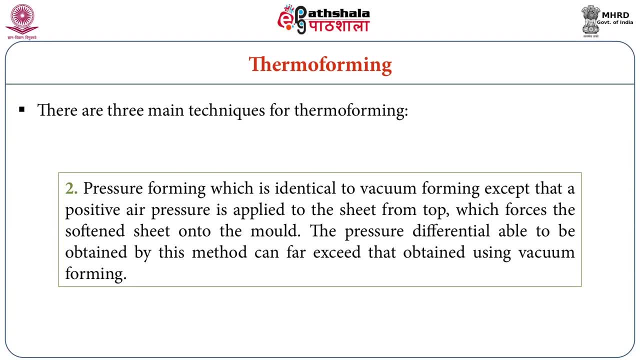 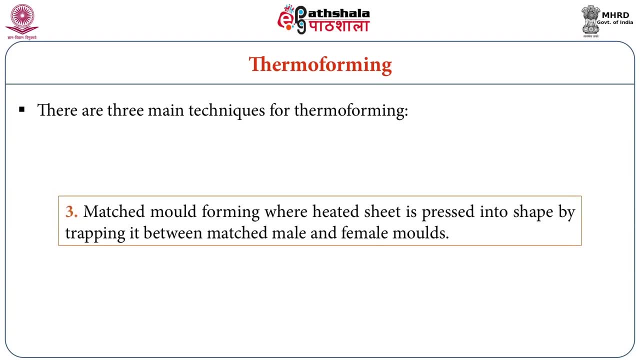 It forces The softened sheet into the mold. The pressure differential able to be obtained by this method can far exceed that obtained using vacuum forming. Third one is matched mold forming, where heated sheet is pressed into shape by trapping it between matched male and female molds. 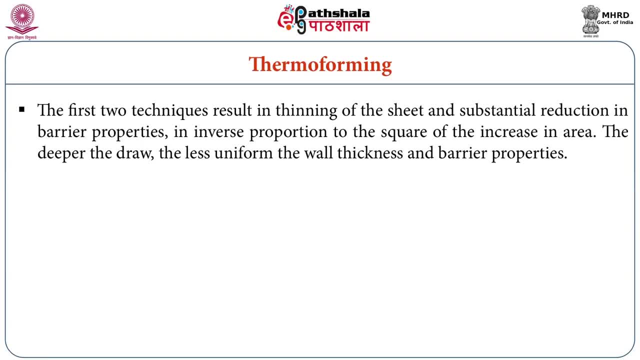 The first two techniques results in thinning of the sheet and substantial reduction in barrier properties In inverse proportion to the square of increasing area. The deeper the drop, the less uniform the wall thickness and barrier properties. Thermally stable PET containers are common for dual oven able applications for chilled 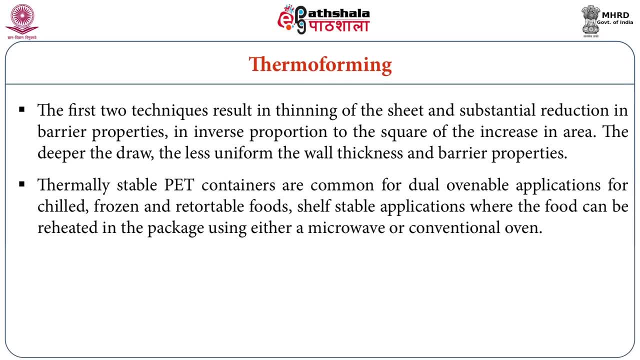 frozen and retortable foods. Self-stable applications where the food can be reheated in the package using either a microwave or conventional oven. These containers are known as crystallized PET or CPET and are able at temperatures up to 230 degree centigrade. 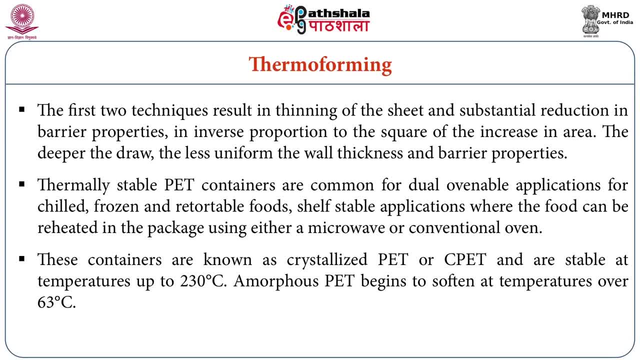 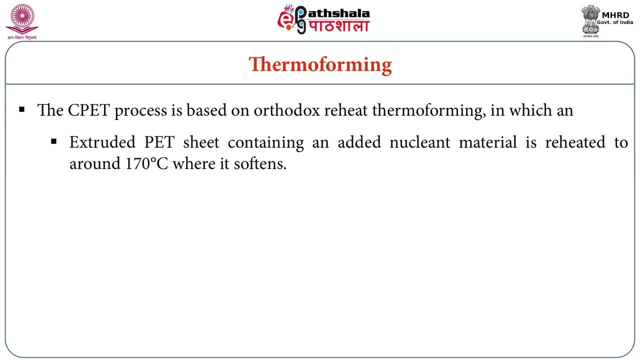 Amorphous containers are known as crystallized PET or CPET and are able at temperatures up to 230 degree centigrade. Amorphous PET begins to soften at temperatures over 63 degree centigrade. The CPET process is based on orthodox reheat thermoforming, in which an extruded PET sheet 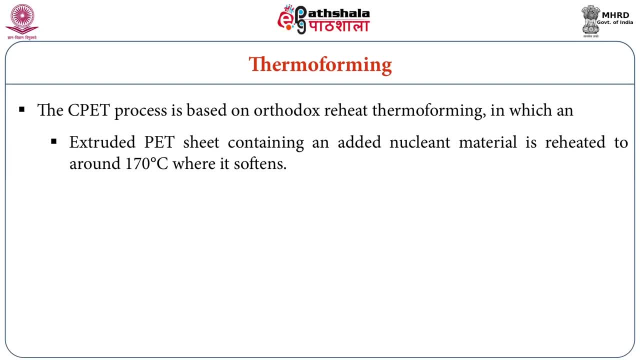 containing an added nucleant material is reheated to around 170 degree centigrade, where it softens. It is then thermoformed into hot mold and held for a crystalline structure to develop for long period. It is then transferred into second mold where it is re-heated. 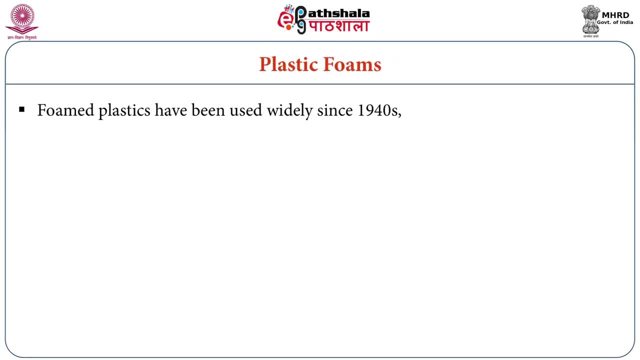 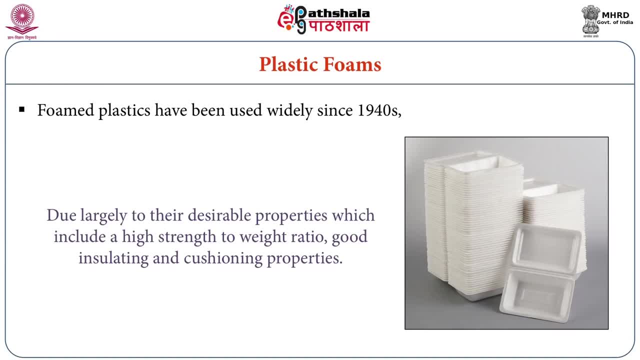 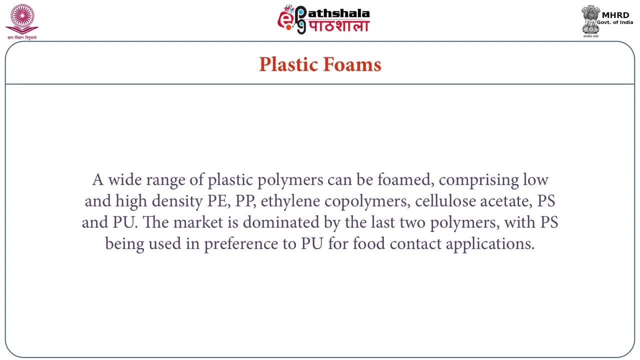 which include a high strength to weight ratio, good insulating and cushioning properties. A wide range of plastic polymers can be formed comprising low and high density: polyethylene, PP, ethylene copolymers, cellulose acetate, PS and polyurethane. 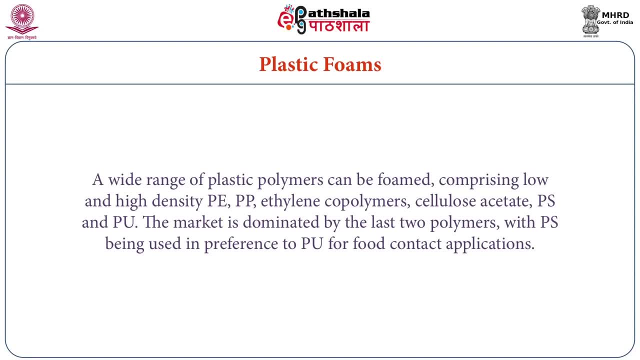 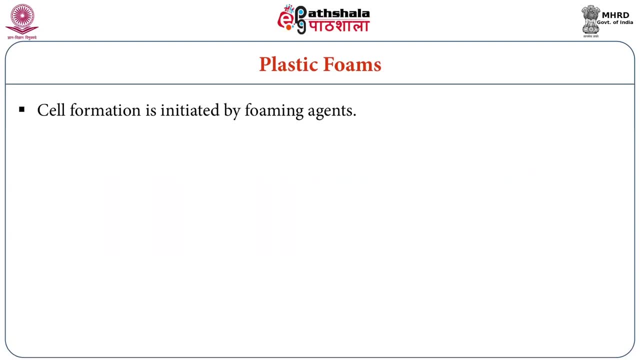 The market is dominated by the last two polymers, With PS being used, With PS being used in preference to PU for food contact applications. Cell formation is initiated by foaming agents. Physical foaming agents are compounds that change their physical state during cell growth. 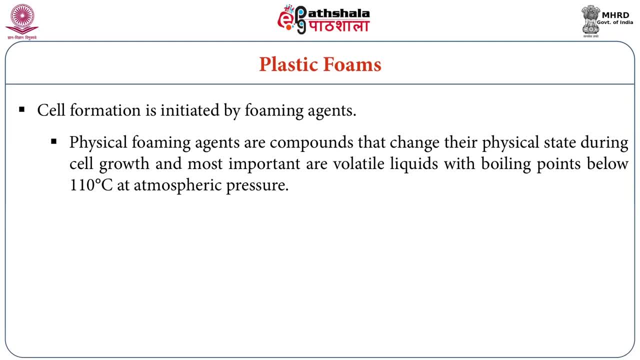 and most important are volatile liquids with boiling points below 110 degree centigrade at atmosphere. Chemical foaming agents decompose under heat: at at least one gaseous decomposition. Chemical foaming agents decompose under heat: at at least one gaseous decomposition. 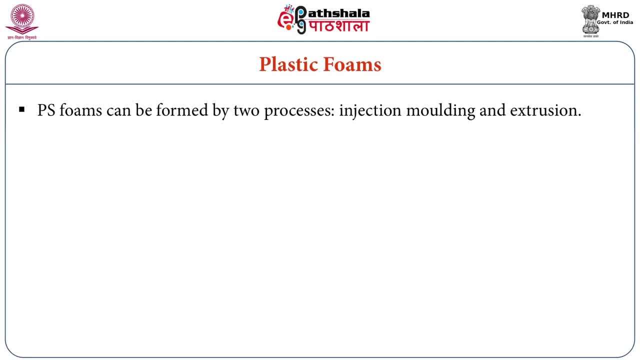 Chemical foaming agents decompose under heat at at least one gaseous decomposition. Usually it is nitrogen. Usually it is nitrogen. PS foams can be formed by two processes: injection, molding and extrusion. PS foams can be formed by two processes: injection, molding and extrusion. 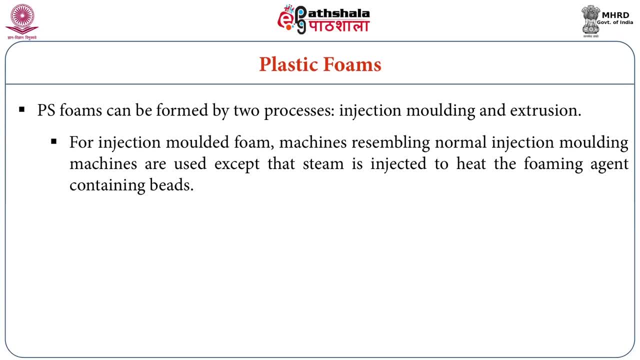 For injection molded foam machines resembling normal injection molding machines are used, except that steam is injected to heat the foaming agent containing beads Extruded PS. foam is produced by free expansion of hot PS blowing agents and additives through the slit orifice of a high strength material. 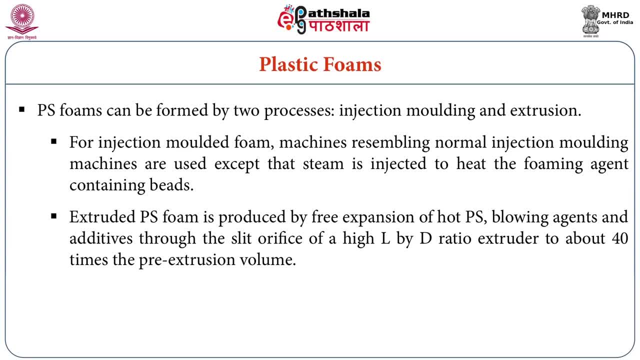 of a high L by D ratio, extruder to about 40 times the pre-extrusion volume. The amount and the type of blowing agent control the density of the foam produced. So to concluding, we can say that there are various methods for conversion and formation. 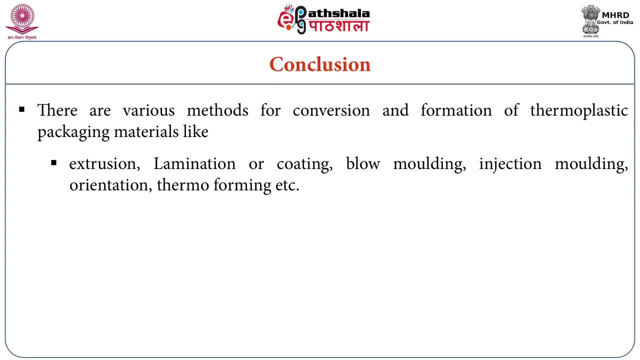 of thermoplastic packaging materials like extrusion, lamination or coating, blow molding, injection, molding, orientation, thermoforming, etcetera. Each method has its typical characteristics, advantages and disadvantages. Research focuses is now on newer methods of thermoplastic conversion. 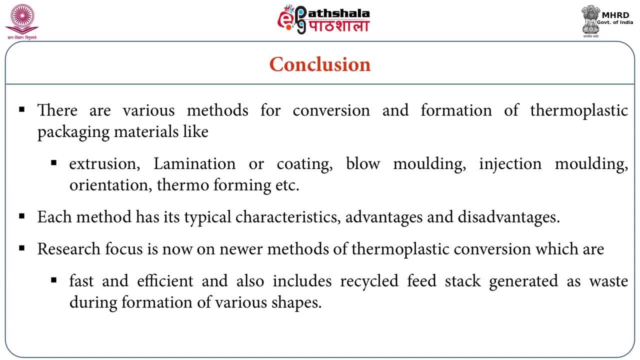 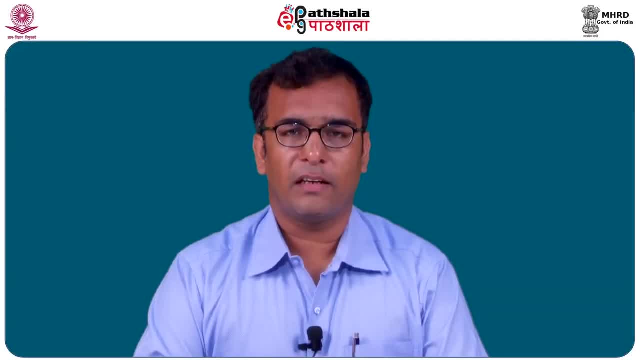 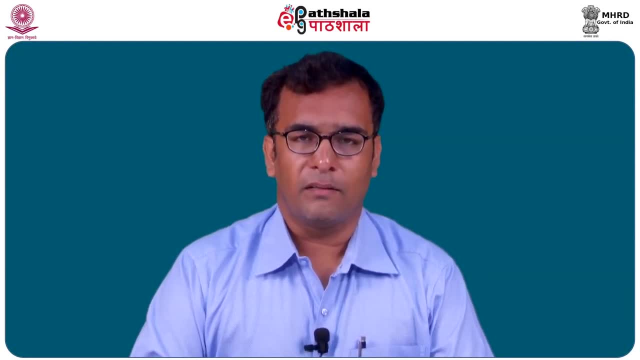 which are fast and efficient, and also includes recycled feed stack generated as waste during formation of various shapes. So, friends, in this module we have learnt about different methods of forming different shapes of plastic materials, which includes thermoforming, injection molding, blow molding, injection blow molding, extrusion and lamination.